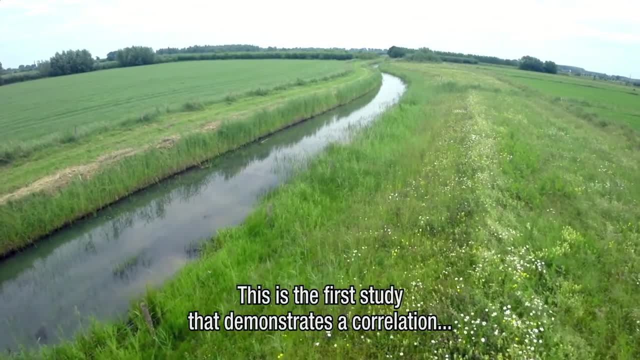 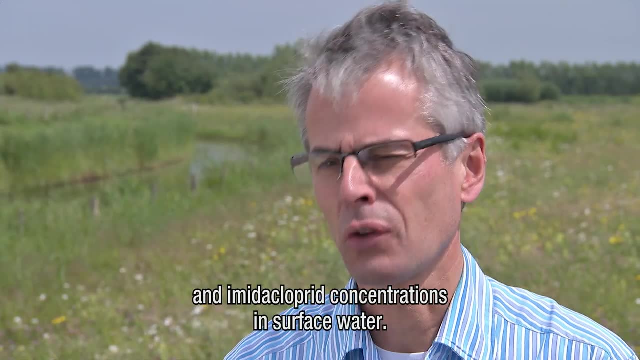 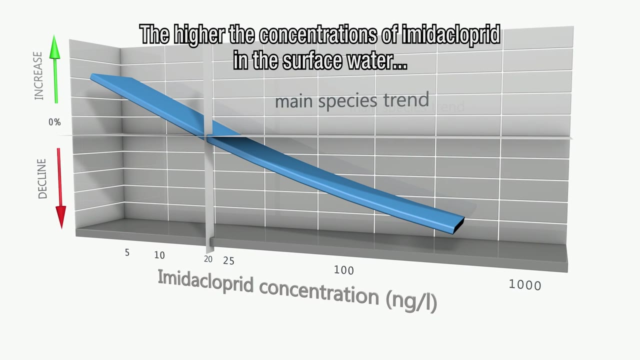 trends between areas. This is the first study that demonstrates a correlation between the decline in populations of vertebrate species and imidacloprid concentrations in surface water. The researchers found a clear trend: The higher the concentrations of imidacloprid in the surface water. 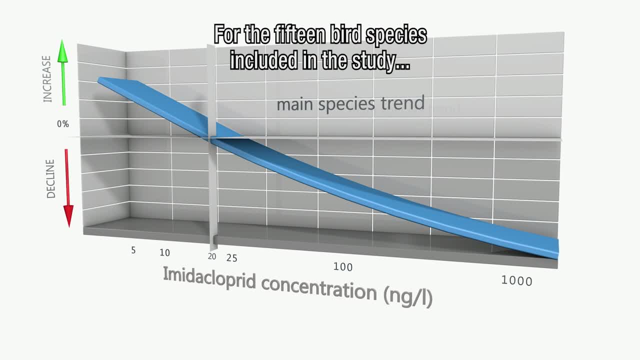 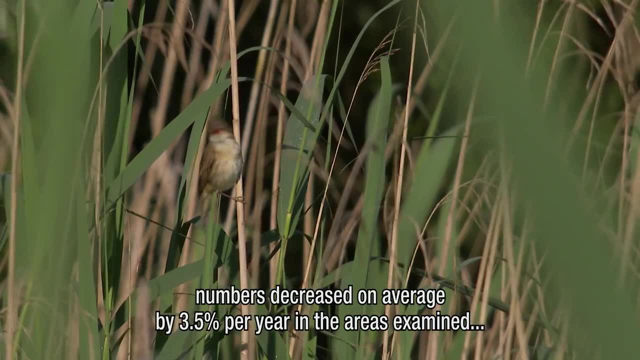 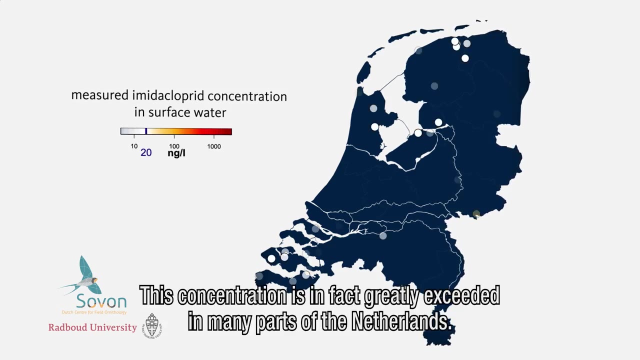 the greater the decline in bird numbers. For the 15 bird species included in the study, numbers decreased on average by 3.5% per year in the areas examined where there was more than 20 nanograms of imidacloprid per litre in surface water. This concentration is, in fact, greatly. 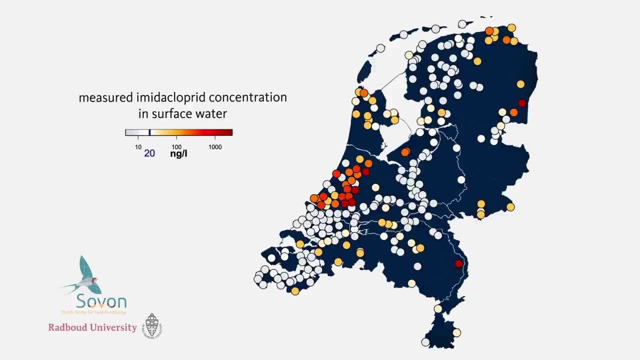 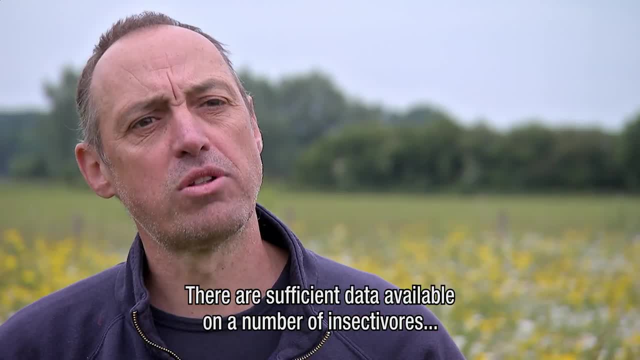 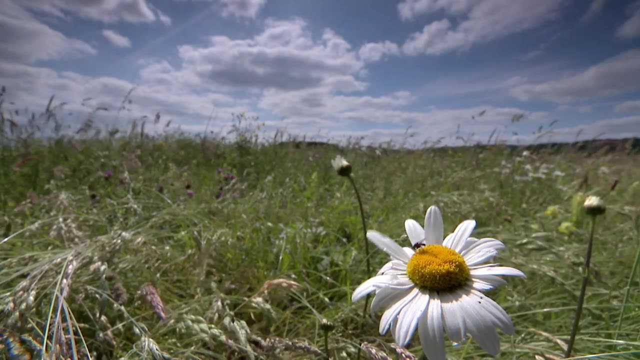 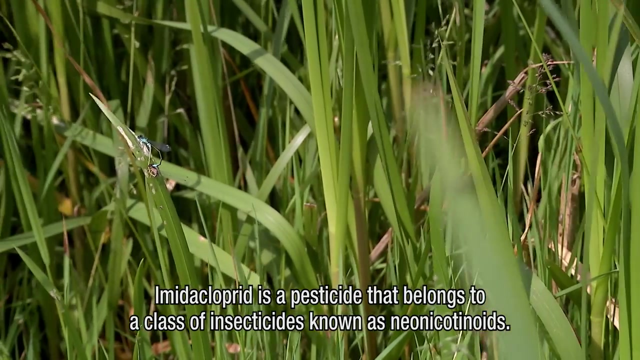 exceeded in many parts of the Netherlands. In many parts of the Netherlands, breeding birds are counted annually. There are sufficient data available on the number of insectivores for us to analyse trends in their numbers in farmland areas. Imidacloprid is a pesticide that belongs to a class of insecticides known as neonicotinoids. 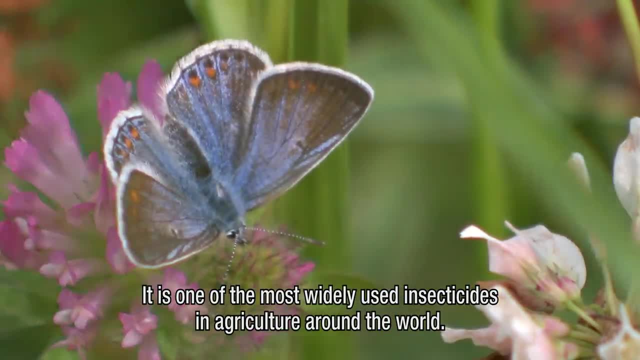 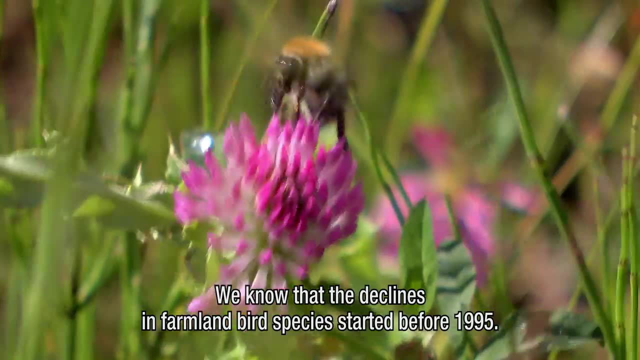 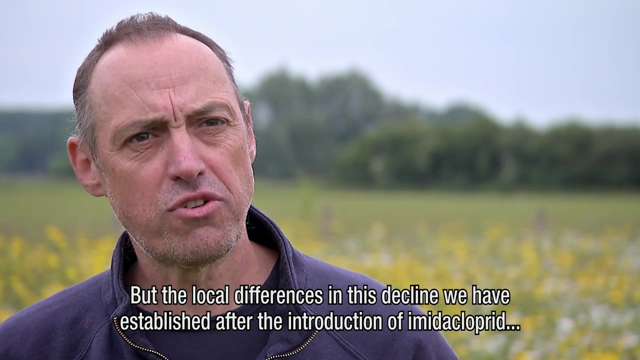 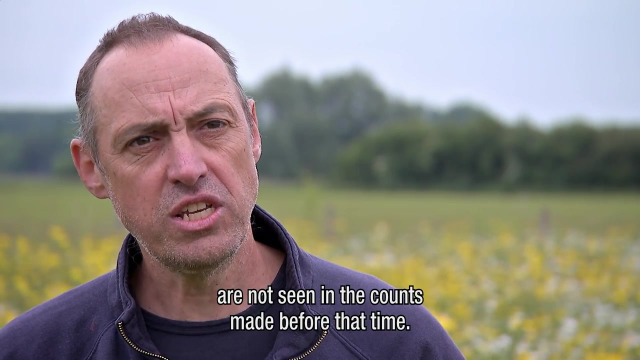 It is one of the most widely used insecticides in agriculture around the world. It was introduced in the Netherlands in 1995.. We know that the declines in farmland bird species started before 1995, but the local differences in this decline that we have established after the introduction of imidacloprid are not seen. 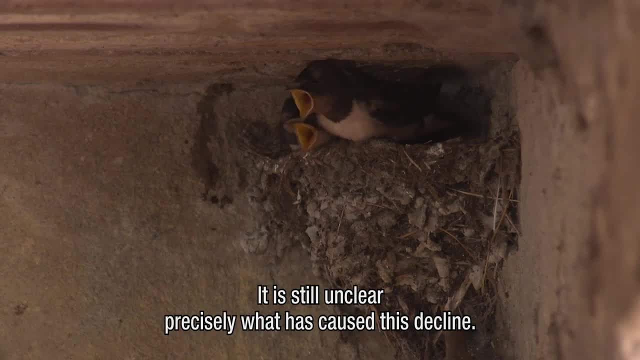 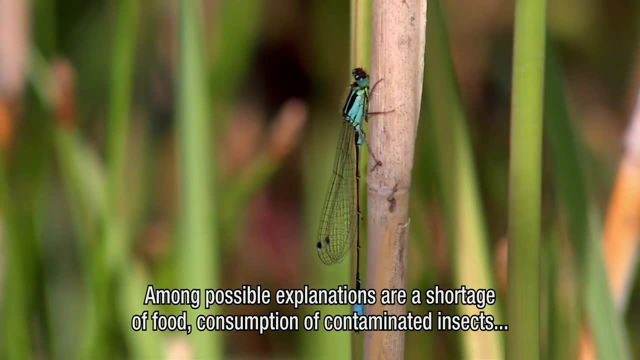 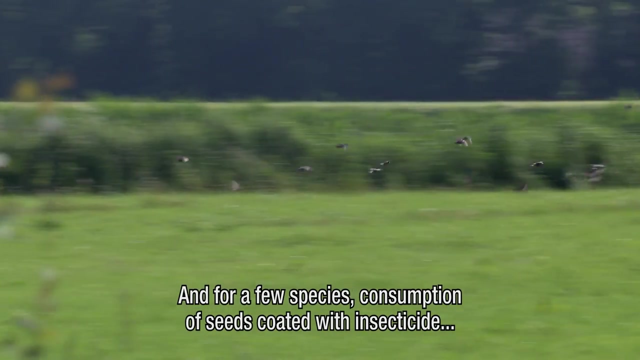 in the counts made before that time. It is still unclear precisely what has caused this decline. Among possible explanations are a shortage of food, consumption of contaminated insects and a combination of both, And for a few species, consumption of seeds coated with insecticide cannot be excluded as an explanation. 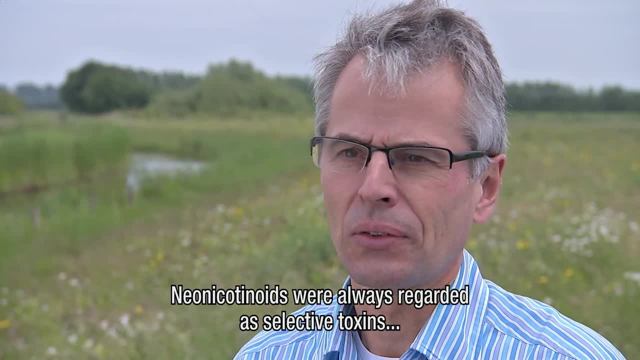 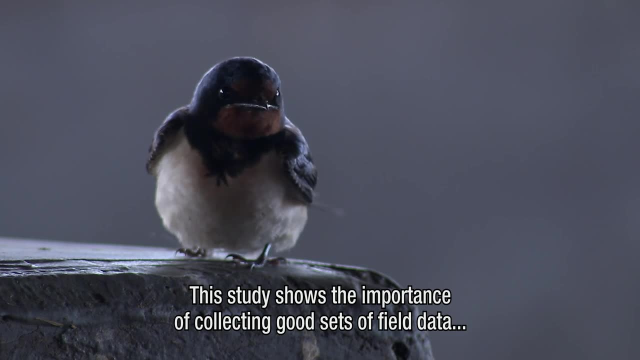 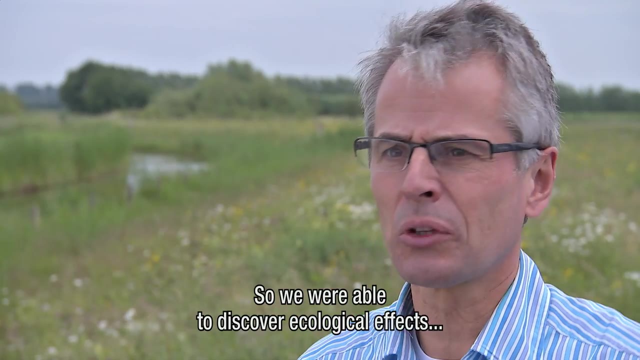 Neonicotinoids were always regarded as selective toxins, but our results suggest that they may in fact influence the entire ecosystem. This study shows the importance of collecting good sets of fuel data and to analyse them in a rigorous scientific way, So we were able to discover ecological effects that would otherwise have been. 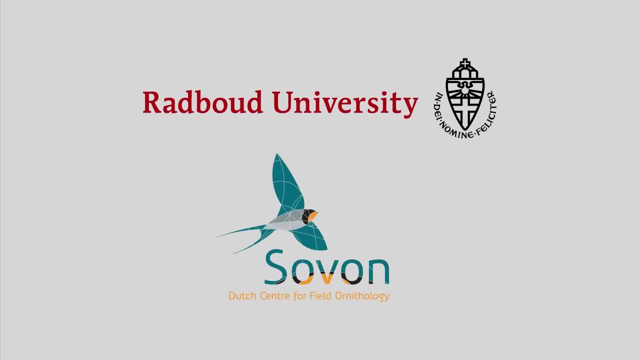 overlooked. Thanks for watching.